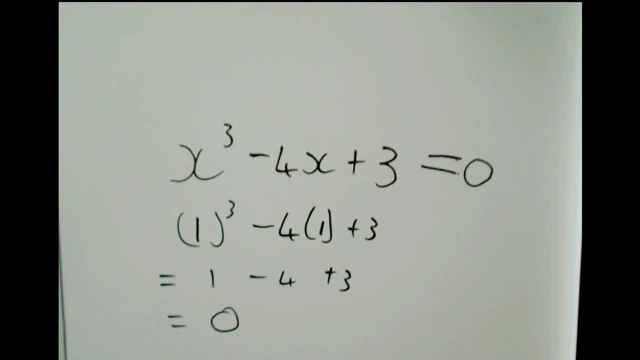 So I know that if I put minus 1 into this side of the equation I will end up with 0. That means that positive 1. 1 is a root. So if this was factorized and positive 1 was a root, we would have the bracket x minus 1 in the solution. 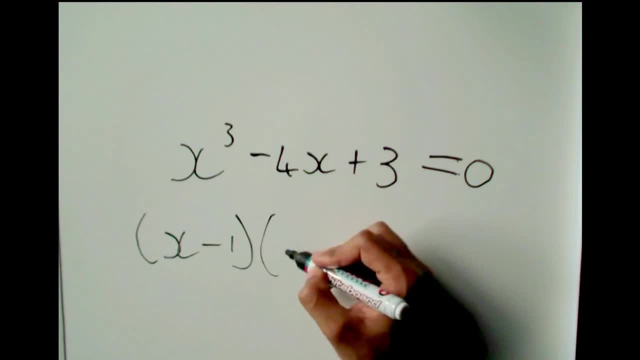 Because- and then we'd have something else here. This would say: x is equal to positive 1, and x is equal to whatever happens in this corner here, Right? So now that we have this factor and we had to guess, there's no better way to do it. 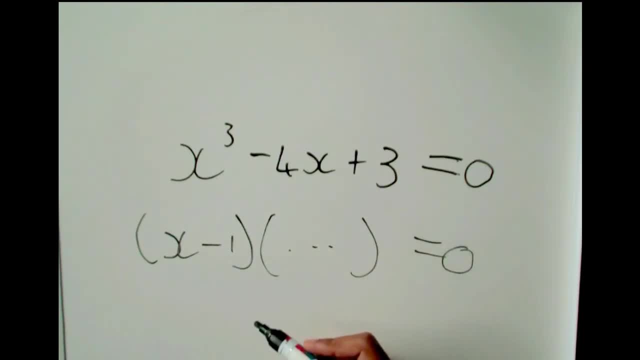 We're going to have to guess a number that works. Now that we have this equation here, we're going to find this, And that's where the kx method comes into play. The other method is dividing out the first factor, but you still need to guess the first factor. 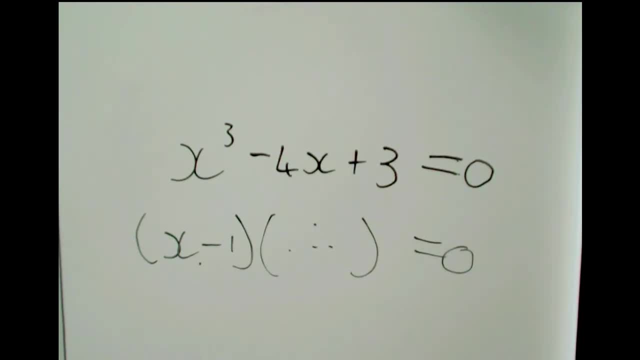 So we're going to find this now. Okay, just remember, this is what we're trying to solve. We will keep this in the back of our mind for now. Just remember, with regular factorization, we're going to find this. 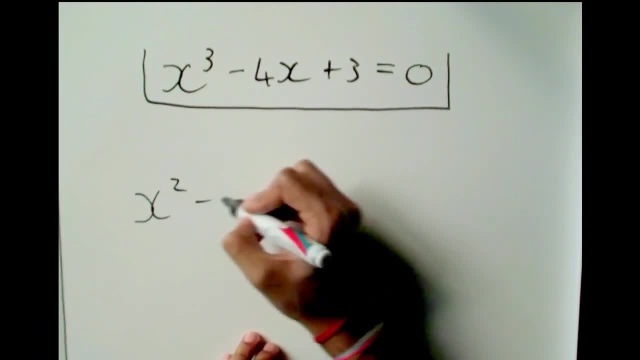 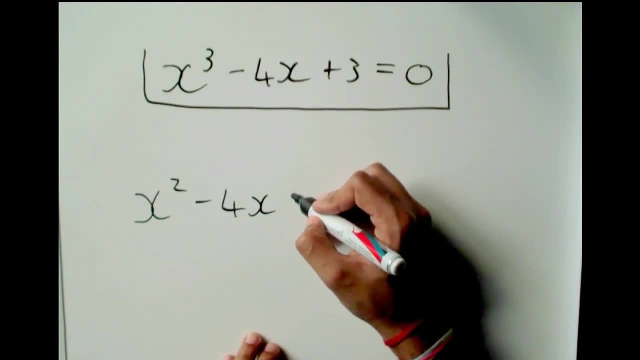 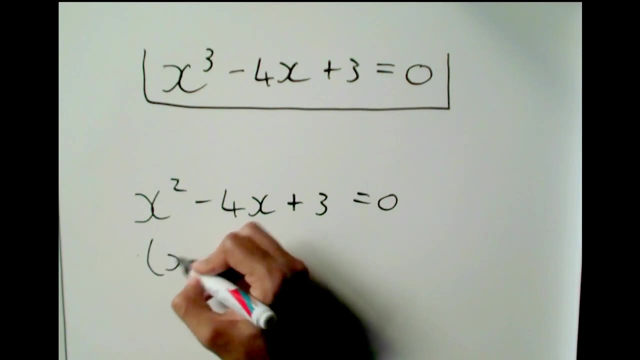 Regular factorization. right, Let's say x squared minus 4x plus 3.. Right, This gives me x minus 3, x minus 1 is equal to 0.. Right, So the regular factorization If I multiply the first number in the one bracket. 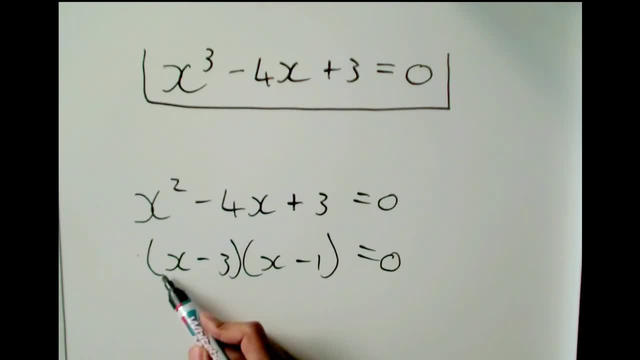 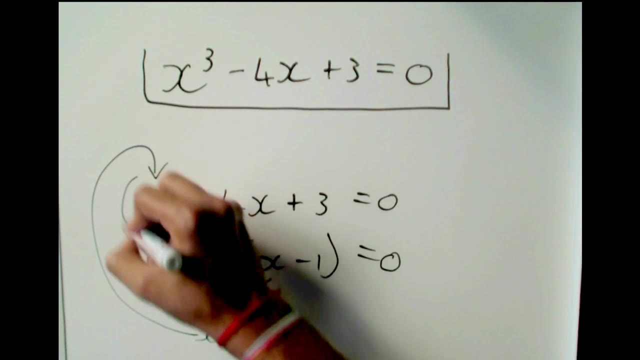 Times. the first, well, the first, if I multiply the first term in the first bracket, the x, and the first term in this bracket, right, this and this gives me x squared, which is my first term, right? So the first term and the first term gives me the first term. 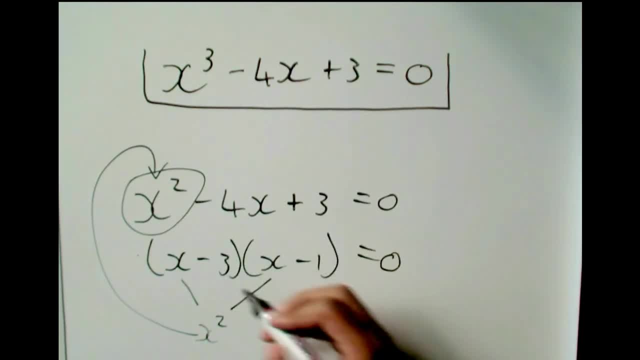 And the same thing happens with the last term. If I took this and this and this, If I take this and I multiply them together, I get 3, which is the same as the last term there. So we know that if we multiply the first term and the first term and the last term and the last term, we end up with the numbers from our original, unfactorized version. 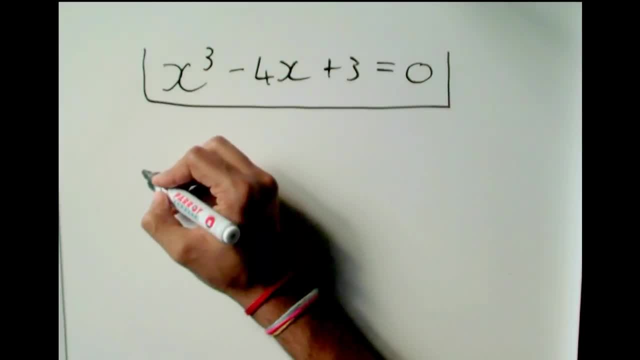 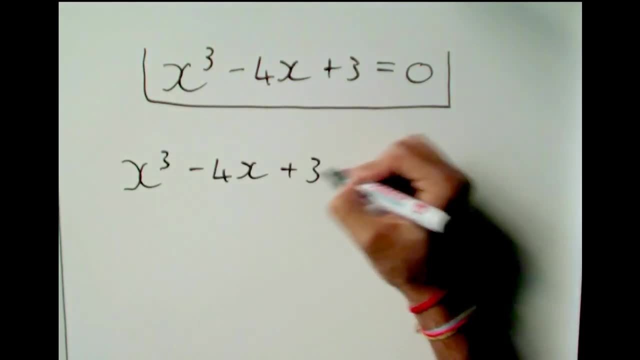 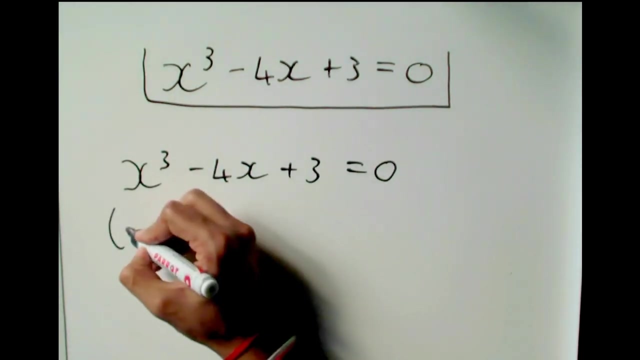 And we will be using this knowledge to do the cubic version. So I already guessed my factor earlier. If you remember, I guessed x minus 1, right Now my next bracket. I do not know what my next bracket is right. 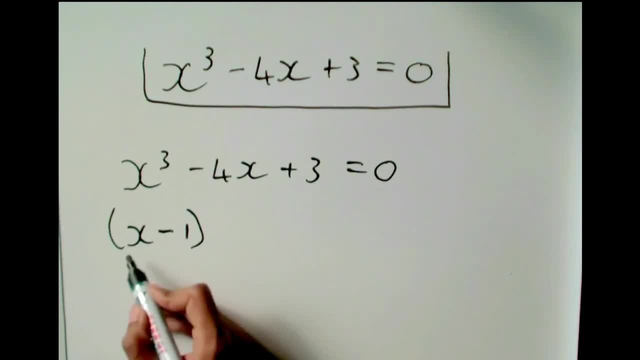 But I know that the first number in my next bracket times the first number in this bracket, must give me that first term, x cubed. So what times, x times. what will give me x cubed? It is x, It is x squared. 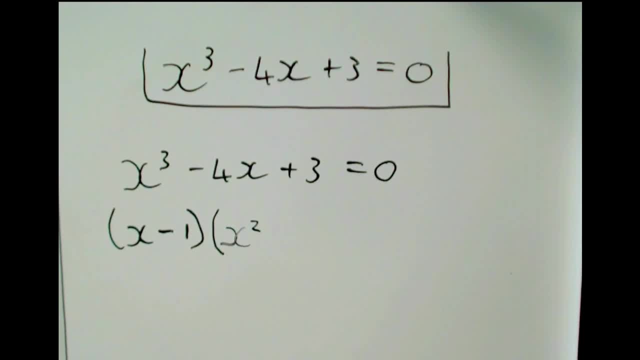 Right, This middle term I do not know about. So what I am going to do is I am going to give it a placeholder. This is why it is called the kx method. I am going to call that kx. I know it should be an x, because it will be an x squared plus something, x plus something. 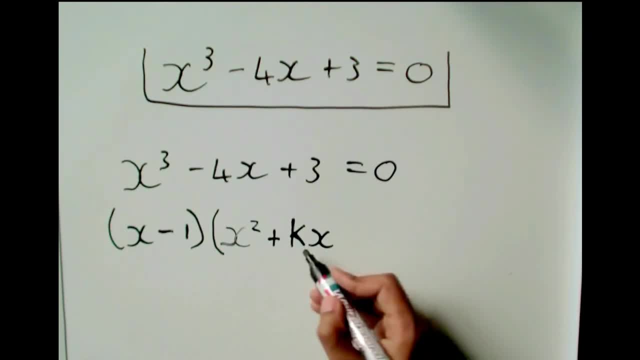 But I do not know what kx, So I am going to call it k for now And I am going to find out what it is later. But the last term I do know- I know that this number times the last term- must give me the last number. 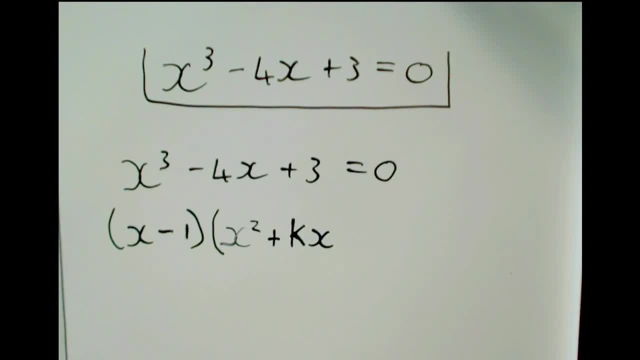 As explained in the squared case In the case earlier. So minus 1 times what will give me 3?? It will give me minus 3.. Okay See. So x times x squared will give me x cubed, And minus 1 times minus 3 will give me 3.. 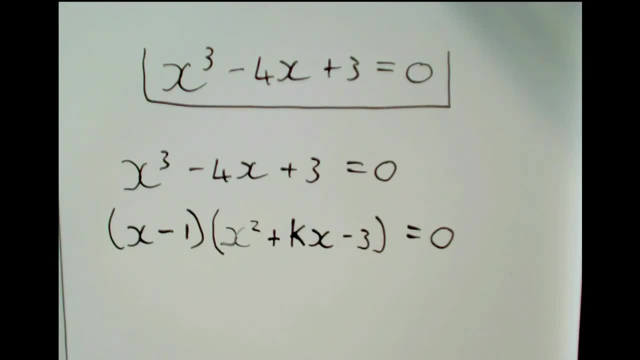 That is how we got these two numbers over here. The middle term we do not know. So let us multiply this guy out. We do not have to multiply the whole thing out when you are doing the method, But for explanation purposes you will see what happens when you multiply the whole thing out. 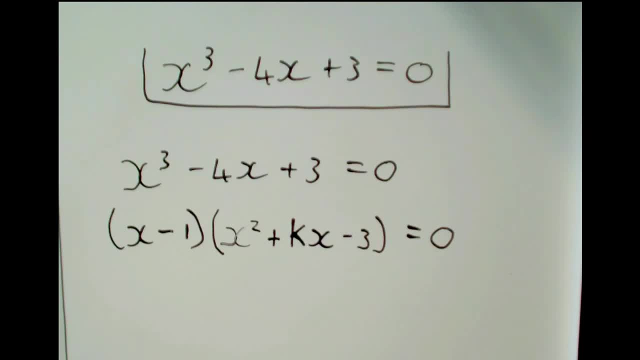 What we are trying to do is find out what k is. So, multiplying this out, we will get: x times x squared will give me x cubed. Then x times kx will give me plus kx squared. And then x times minus 3 will give me minus 3x. 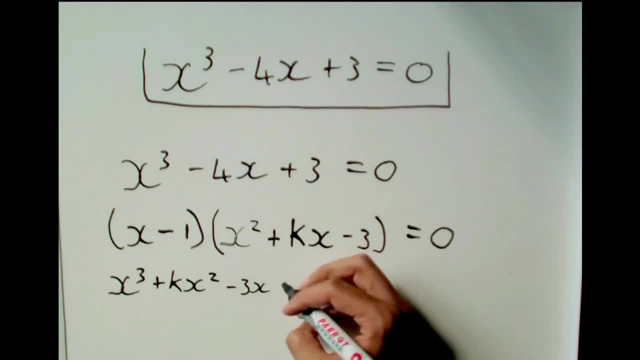 Now, minus 1 times x squared gives me minus x squared. Minus 1 times kx gives me minus kx, And minus 1 times gives me plus 3.. Equals 0. So we need this to be the same as this. 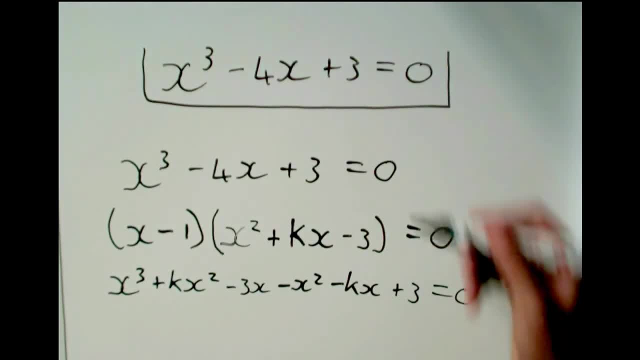 For the equation to work, Because that is what we started with. After we factorize and multiply out, we should end up with what we started with. That is how we are going to find out what k is. We are going to see: I have minus 3x plus kx. 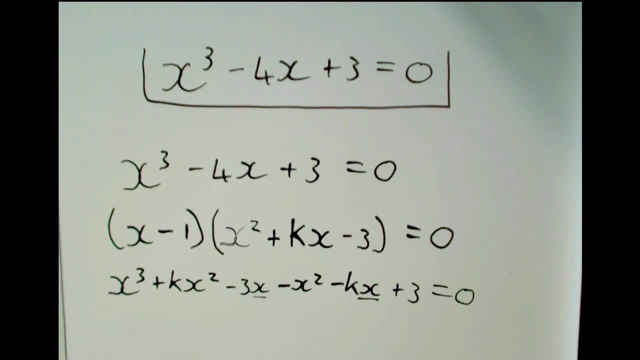 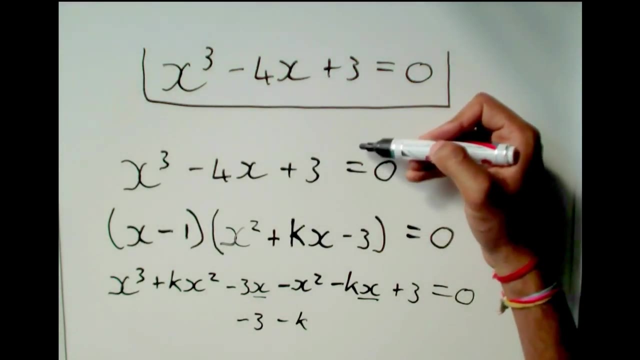 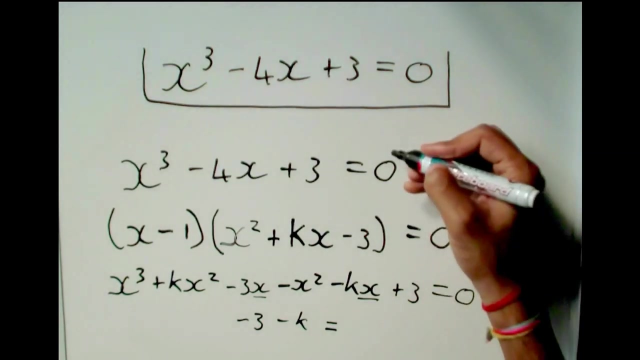 So from the x term I have minus 3 minus k. I have minus 3 minus k x's Right In my expanded out version And in my original version I have minus 4 x's. So these should be the same, if this equation has to be the same as this equation. 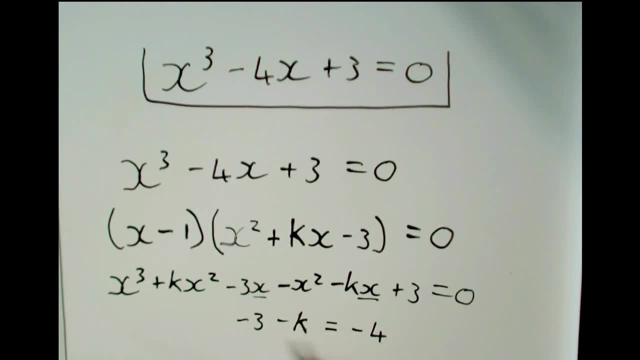 And now, if I solve this by taking this 3 across, I end up with minus k is equal to minus 1.. So k is equal to 1.. So k is equal to 1.. Now that we have the value of k, 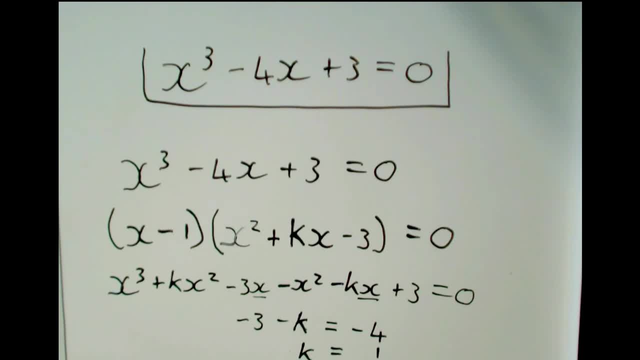 We just need to substitute it into here And then we will factorize that last piece to get our fully factorized version. Another way I could have done this is We don't look at the x term Right, We could also have looked at the x squared term. 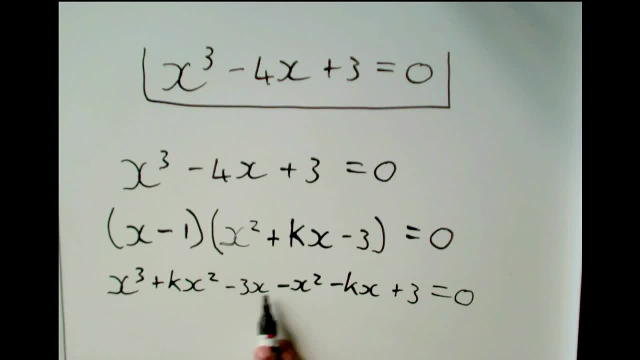 The x squared's. I have kx squared's Minus 1 x squared. So I have kx squared's Minus 1 x squared's, And that must be equal to how many x squared's we had originally. 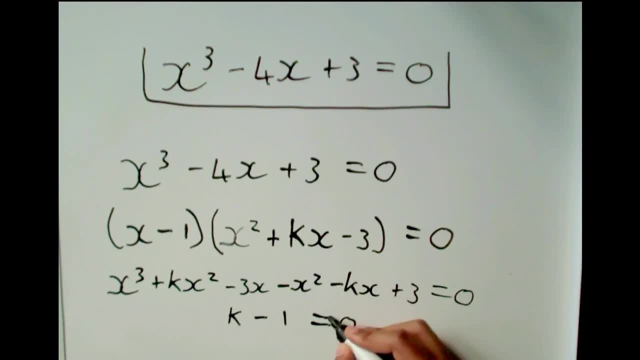 And originally I don't have any x squared's, So I have 0 x squared's Right And in taking the 1 across I end up with k is equal to 1. As before, And these must be the same thing. 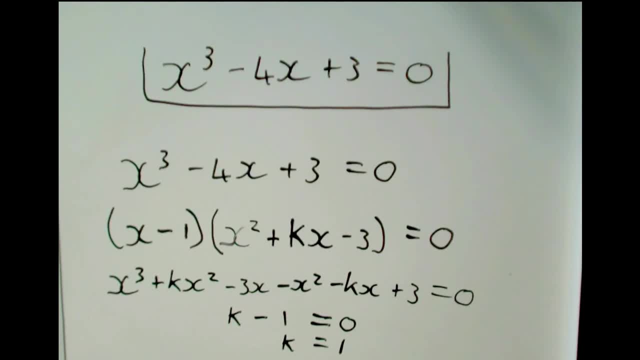 If they are not the same thing. If you want to do a quick check for yourself, If you want to make a mistake somewhere, You can check that using the x squared's or using the x's must give you the same value of k. 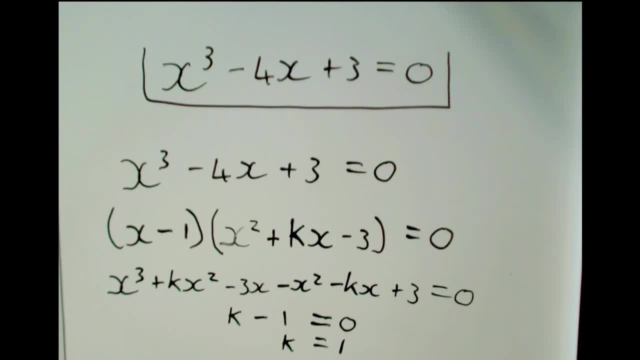 And if they don't, You have made a mistake somewhere And you can go check if you didn't multiply a negative out correctly, or something like that. So now that we know what k is, We can go. We can go here. 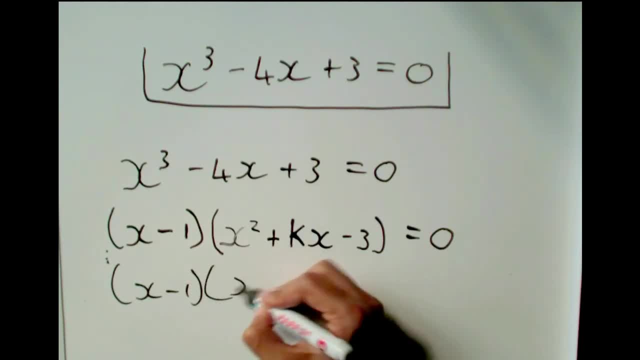 And we can say: this is x minus 1.. x squared plus x- Because I am putting k as 1 in there- Minus 3 is equal to 0.. So here we have the fully factorized version. I say fully factorized because in this case this term does not factorize. 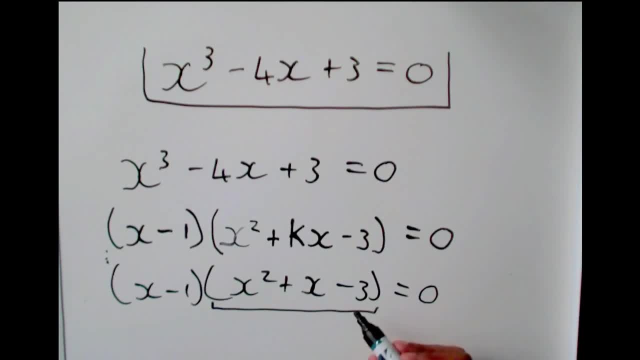 So if this was, let's say, a 2. If there was a 2 here, Then we would be able to factorize this, And we would have to factorize it to get our answer. So, because that doesn't factorize, 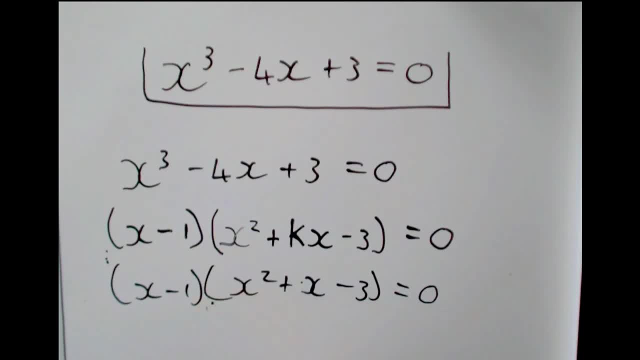 Our answers are: x is equal to minus 1.. Or positive 1, sorry. Or x is equal to Something out of the quadratic formula From this. So I would have to say: Minus b plus or minus root b squared minus 4ac all over 2a. 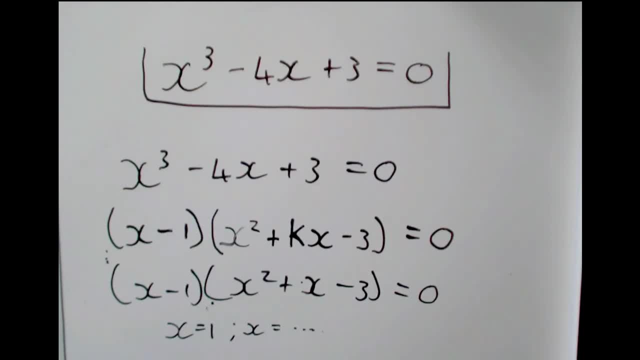 To get those, To get those answers And I end up with 3 answers. We expect to get 3 answers, Because we were working with a cubic function. It is possible- It is possible that we get less than 3 answers. 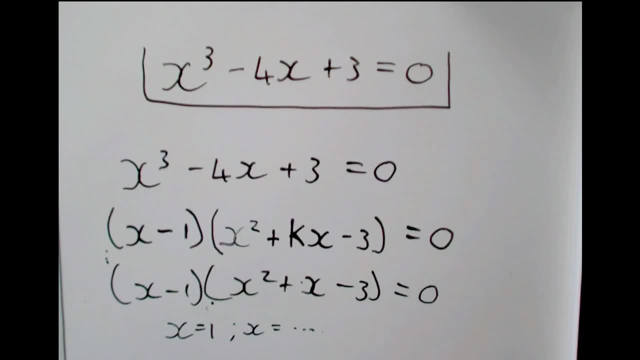 Because we could have a bracket that is squared And then you would end up with the same answer twice. But we can't get more than 3 answers Because that is the maximum we can get with a cubic function. I hope you all now know how to factorize polynomials of degree 3.. 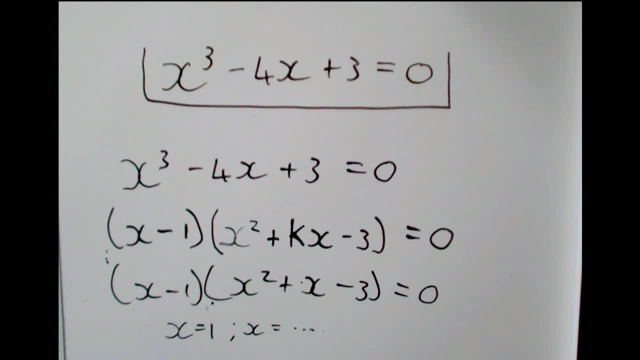 So cubic polynomials. Feel free to check out the other video Where we learn how to do it With long division of algebraic expressions. Happy studying.